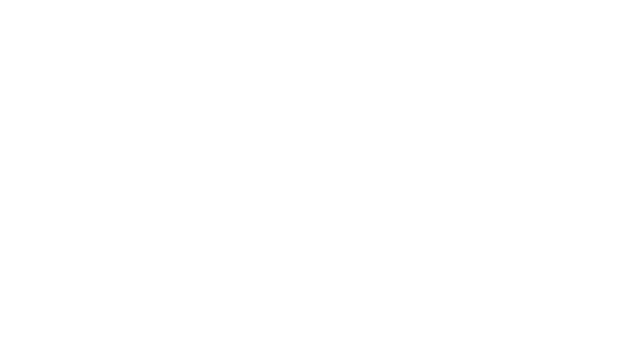 In today's video we're going to cover biotic and abiotic factors, So we'll discuss what each of them are and then we'll take a look at an actual ecosystem and try to spot the relevant factors there. We can describe biotic factors as any living factor that affects another organism. 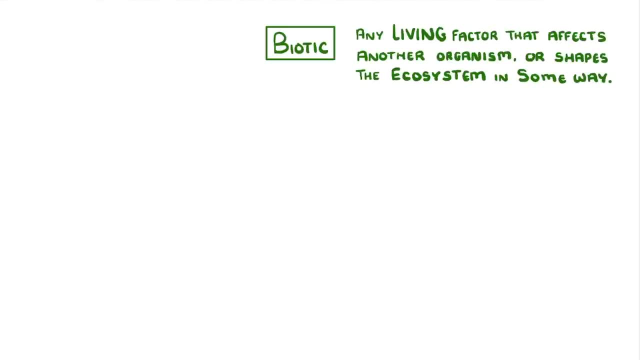 or that shapes the ecosystem in some way. It's kind of a hard one to describe, but if you think of something like predation, then we would class that as a biotic factor, because it's a living process and it can influence the population of another species, In this case, whoever's leg that 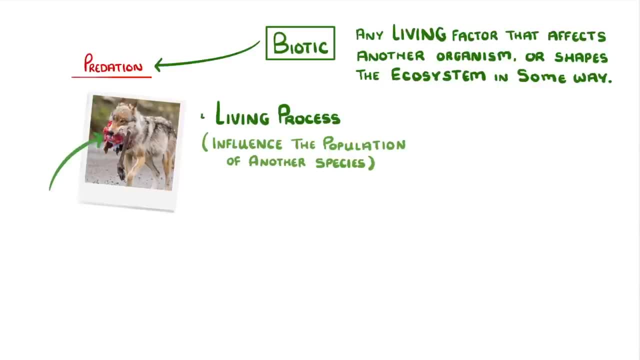 was. Other biotic factors would be things like competition for resources or habitat, the amount of disease and the availability of food. So if you're asked to find the biotic factors in an ecosystem, just think of all the ways that the living organisms, whether they're animals, plants, bacteria or anything else that's living- 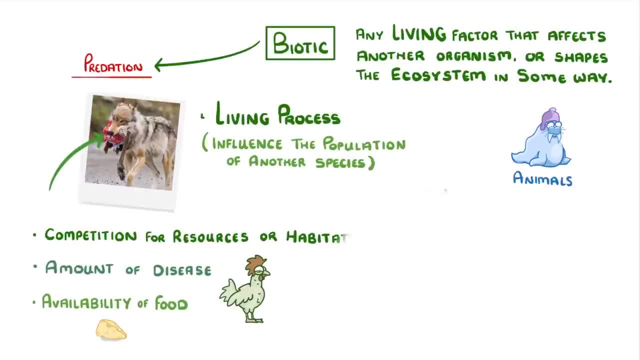 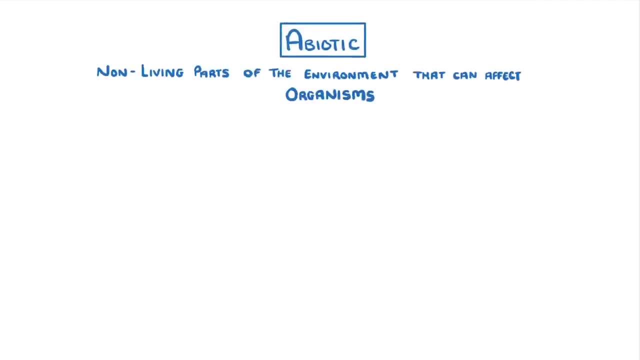 can affect one another. Abiotic factors, meanwhile, are all of the non-living parts of the environment that can affect organisms, So these are often the chemical or physical parts of the environment. It includes things like the light intensity, temperature, carbon dioxide concentrations. 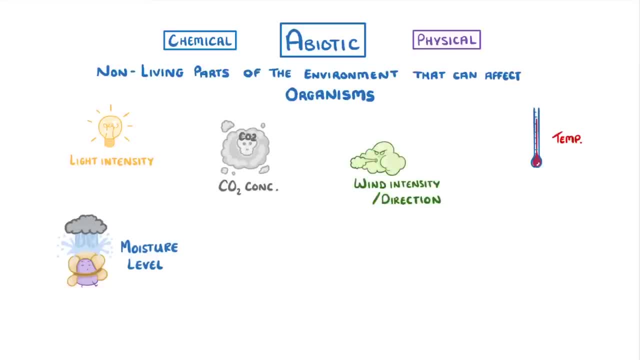 moisture levels, the intensity and direction of the wind and the pH and mineral content of the soil. So if we were to pick any one of these, we could hopefully explain what impact changing it might might have on the environment. For example, an increase in temperature could. 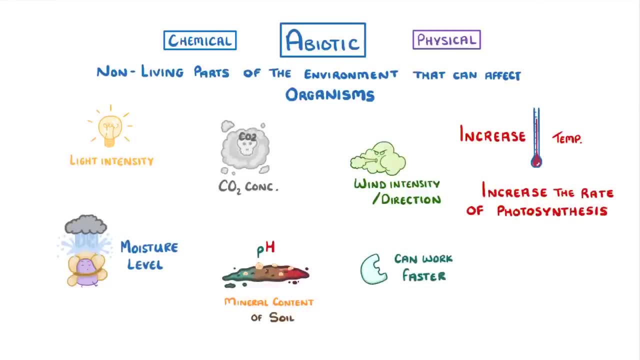 increase the rate of photosynthesis because the enzymes involved can work faster, and so, as a result, there might be an increase in the overall rate of energy plant growth. It could also mean that animals have to spend less energy staying warm, so they might be able to use more energy for growth or spend less time searching for food. 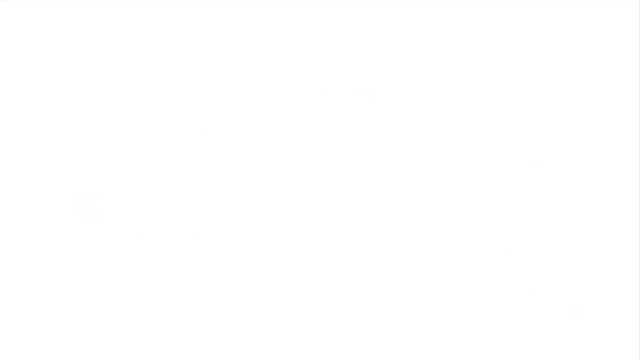 Now, typical questions for this topic will generally focus around identifying these various biotic and apodic factors and then trying to explain what will happen if they change. So if you think about a clownfish chilling out by its sea anemone, what would be the main biotic and apodic factors that affect it?